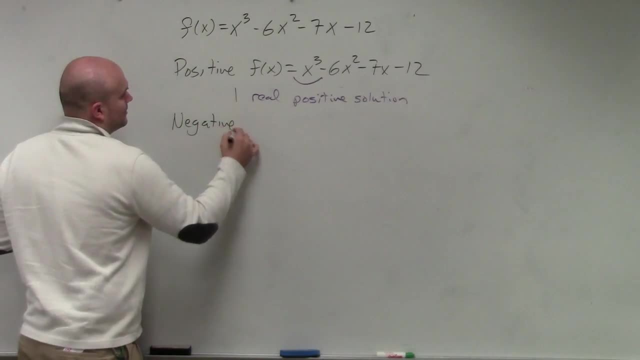 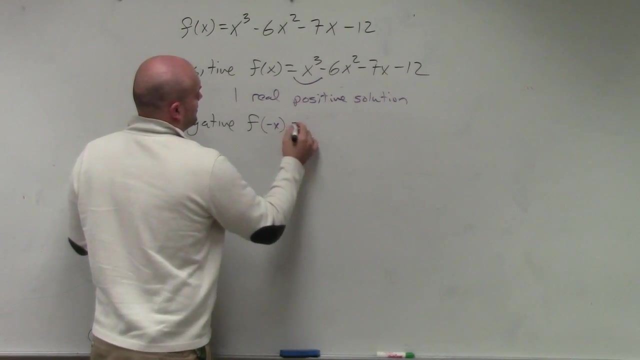 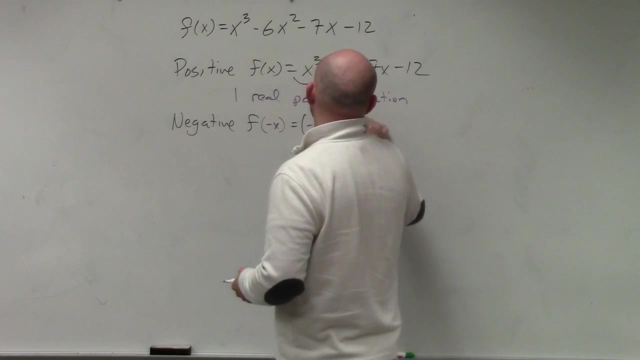 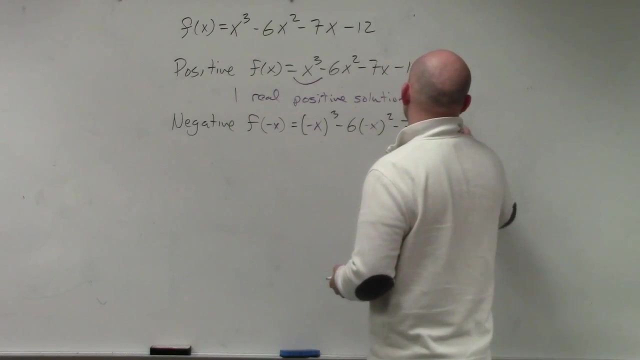 The negative involves a little bit of work. So the negative: you need to do f of negative x. So when you're doing f of negative x, you have negative x cubed minus 6 times negative x squared minus 7 times negative x minus 12.. Is everybody okay with that step? 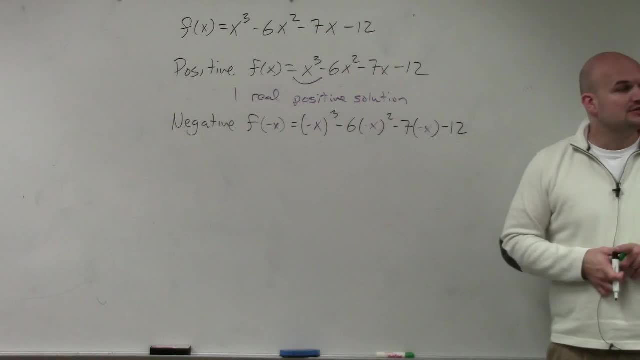 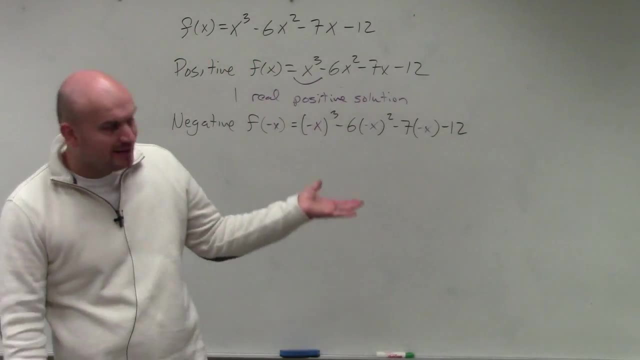 Speak now or forever. hold your peace, Everybody's okay. Just remember, guys: whenever you have a negative value raised to an odd power, it's still going to be negative. Whenever you have an odd value raised to an even power, it's going to turn positive. So negative x cubed. 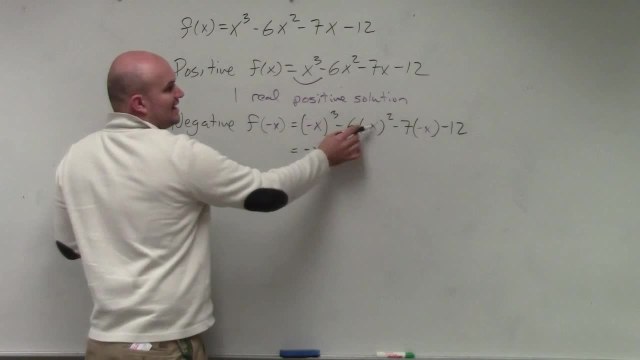 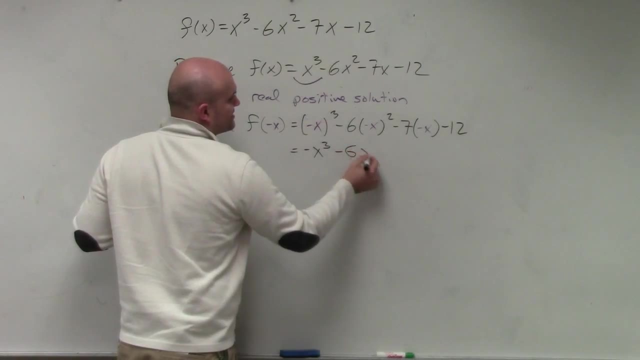 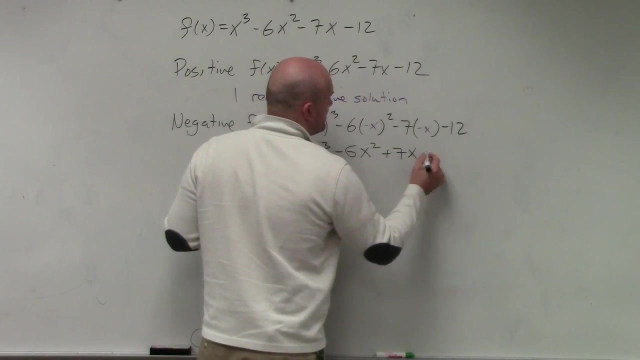 is going to now turn into negative x cubed. Negative x squared is now positive x squared. But positive x squared times negative 6 is now a negative 6 x squared. Negative 7 times negative x is now a positive 7 x minus 12.. So now we count the sign changes: Negative. 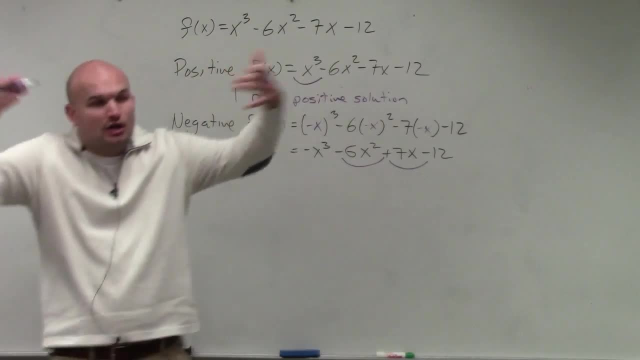 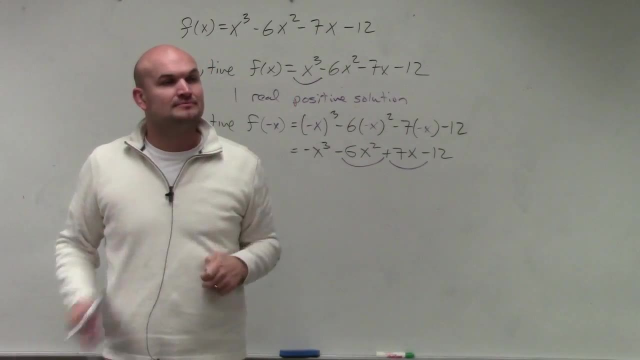 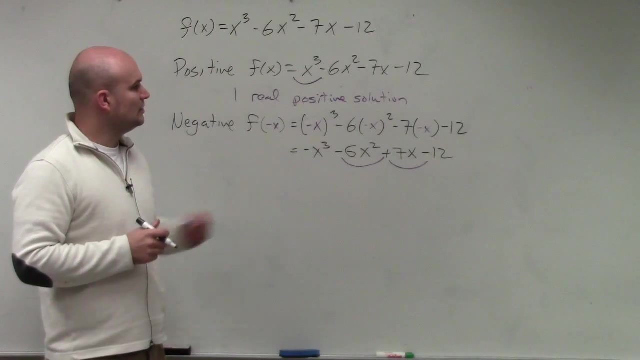 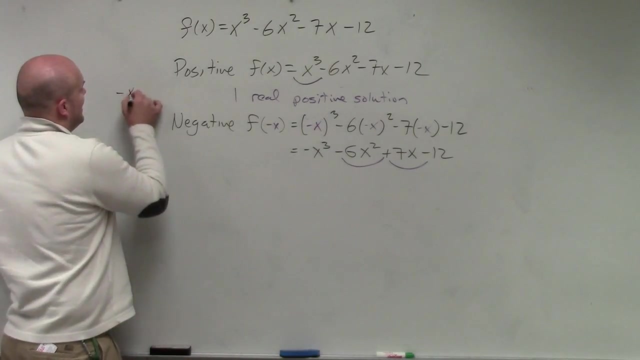 to positive, positive to negative. So remember, Descartes' rule of signs says, though, the number of sign changes minus an even number, Yes, Well, it's a negative 6.. Negative 6.. But remember, it's negative x squared, which is negative x times negative x, Negative x. 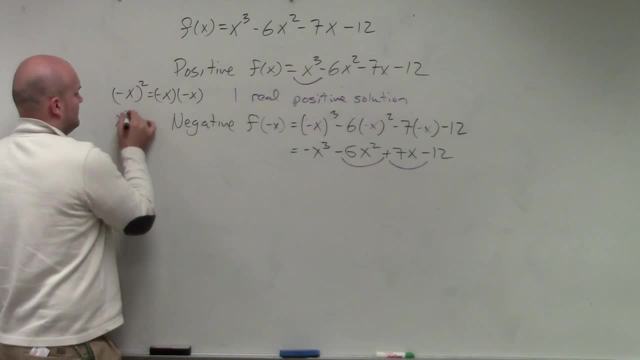 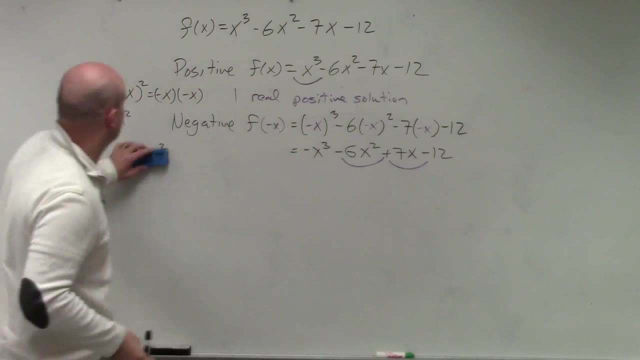 times negative x is what Positive x squared, right. So what's negative 6 times x squared? Just negative 6 x squared. Is that So just the squaring I know it gets. so it's not a time. So just remember any negative number. remember you just use order of operations. 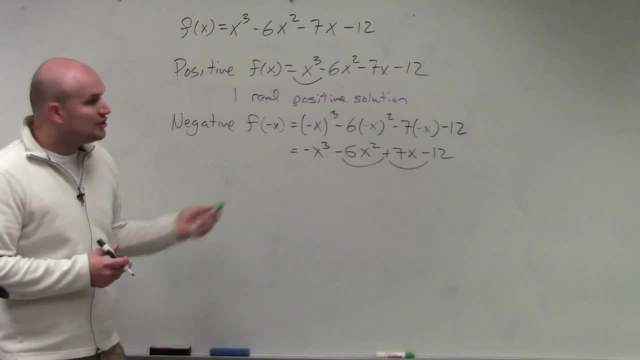 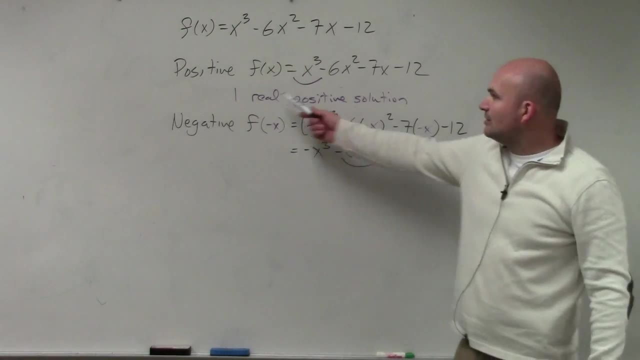 You've got to square it before you multiply it. okay, So it's 2.. But remember Descartes' rule of signs, and this is what everybody forgets: it's always the number of sign changes minus an even number. Well, I can't subtract an even number from 1 and 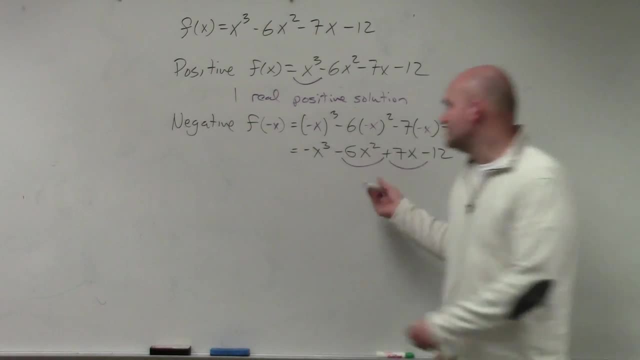 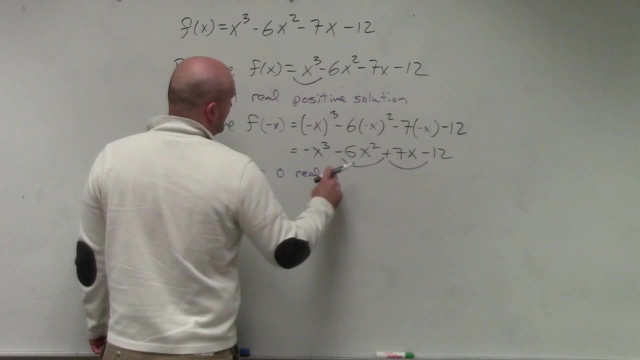 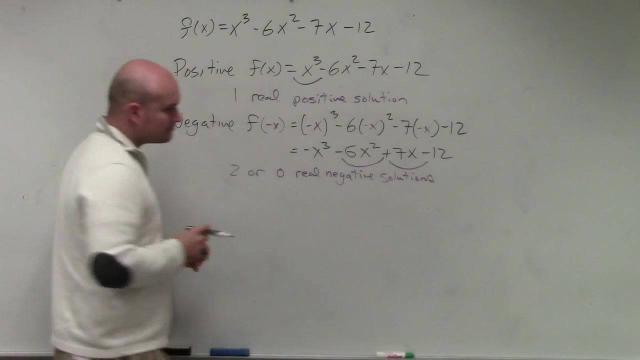 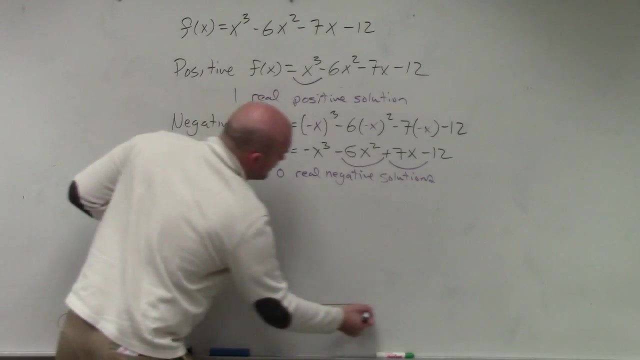 still have a positive value. So I have to subtract. so in this case, I have 2 or 0 real negative solutions or 0s. Yes, Then what I do to find the number of complex is I create my box, which I did in class. 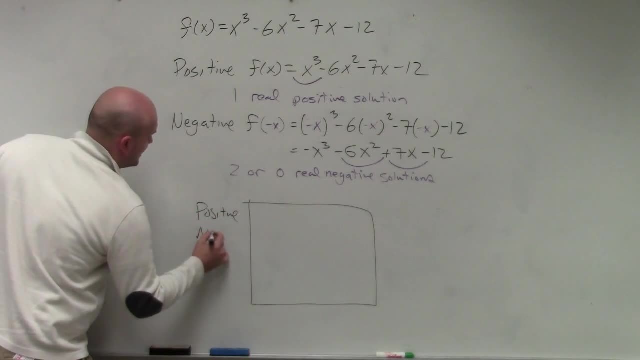 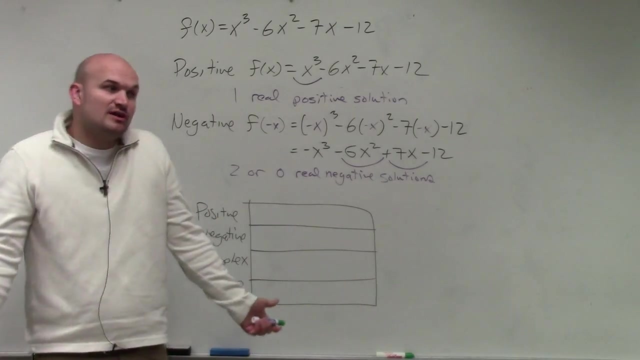 So we do. there's positive solutions, there's negative solutions, there's complex solutions and there's the total, Because I don't know what the question on your test can ask you. so we might as well figure out what all of them are. Well, the number of positive, we 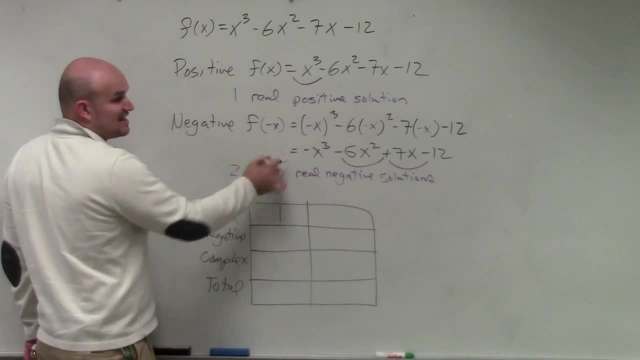 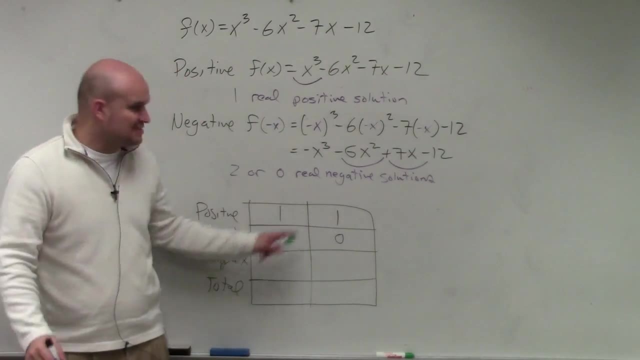 said there's only 1.. What else? Well, the number of negative. there's actually 2 options. You could have 2 negative or you could have 0 negative, right? So I know that? for since my negative has 2 options, 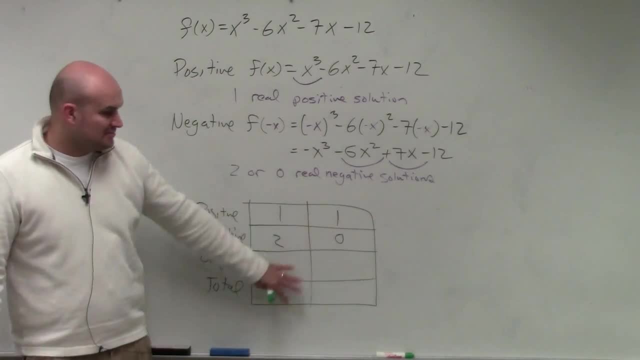 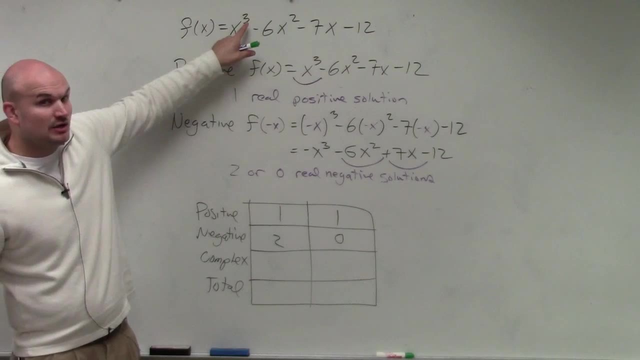 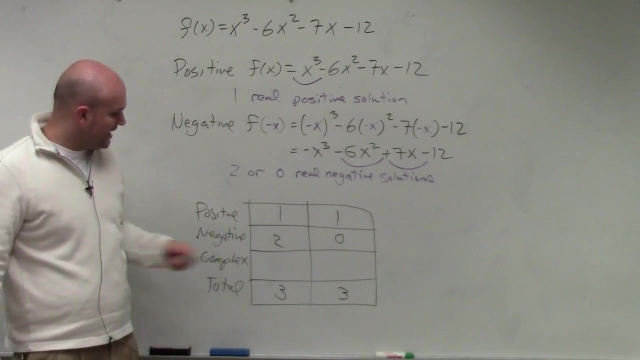 that's why I created 2 rows for each option, or 2 columns for each option. Well, positive is always 1.. Negative is 2 or 0. The total is the degree right. You can only have as high as your total, and that's going to be 3 and 3.. Well, if I have 1 positive, 2 negative, 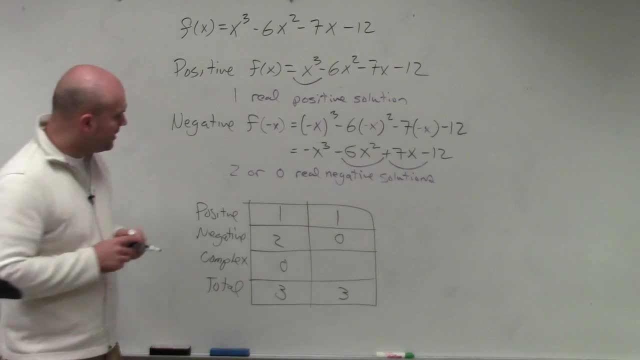 how many complex do I have to have 0.. 0.. If I have one positive, zero negative, how many complex do I need to have to have a total of three solutions, Two. So the total number of complex solutions is two or zero. 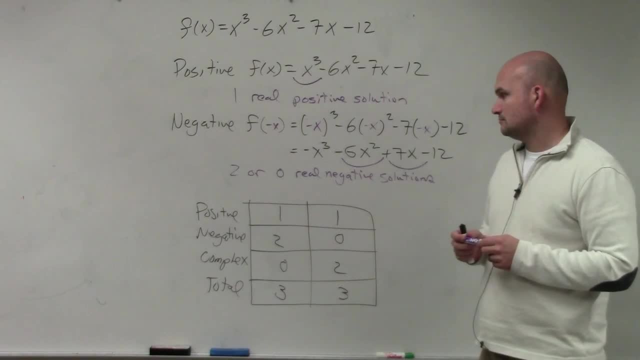 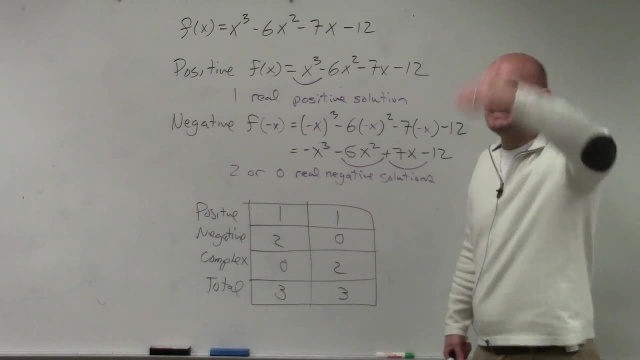 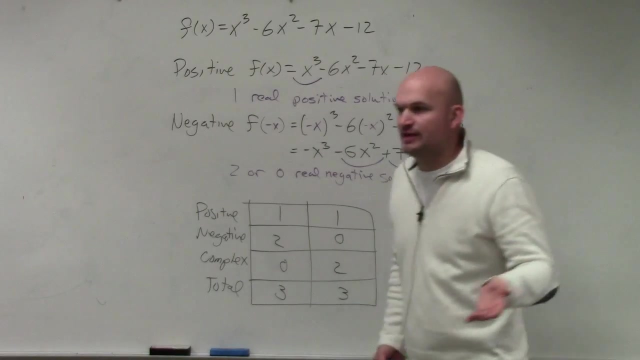 Yes, Can you go over how you got two or zero? That's just the rule of Descartes' Rule of Sines. It states the number of sign changes minus an even number. So I always just subtract two, because when you think of even numbers you think of a number divisible. 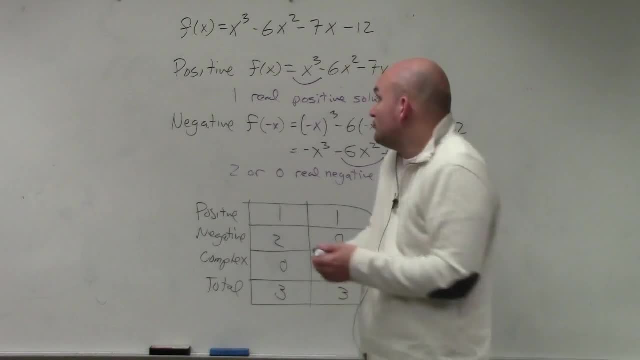 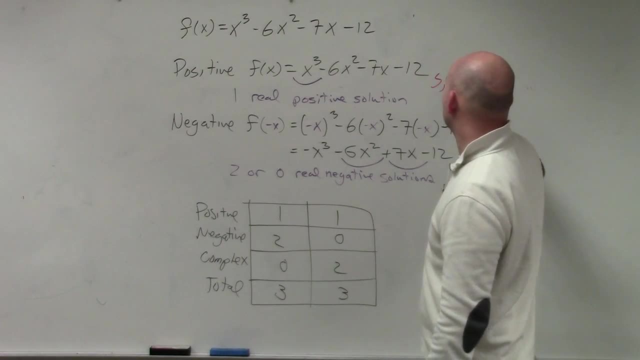 by two. So just always subtract two as many times as you can. So for instance, let's just play a little game. Let's pretend this had five sign changes. Then you do five, three, two, one. Let's pretend it had six sign changes.